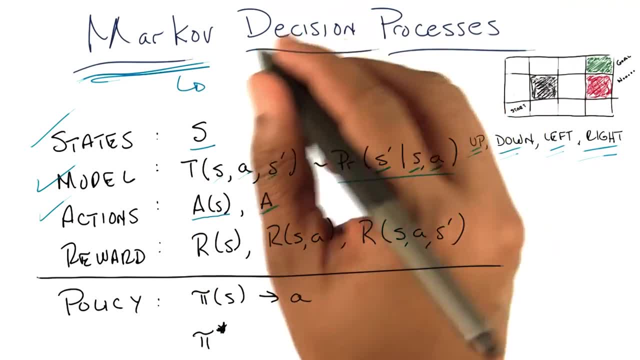 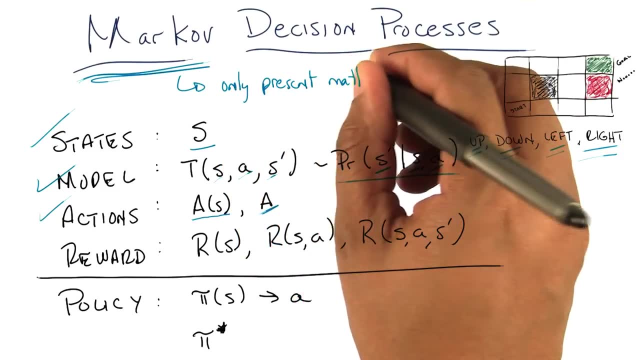 That's exactly right. The Markovian property is that only the present matters, And they had to pass that down to me. you know one generation at a time because you know Markov property. That's exactly right. That's very good, Michael. 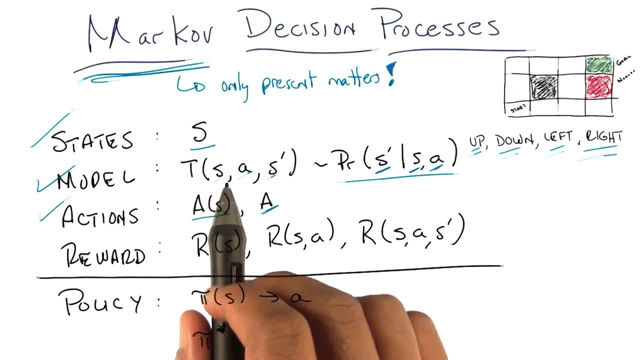 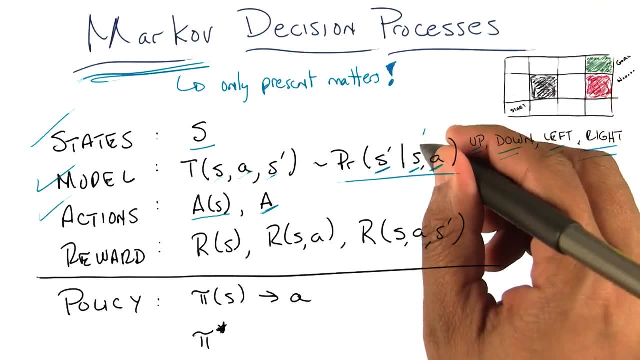 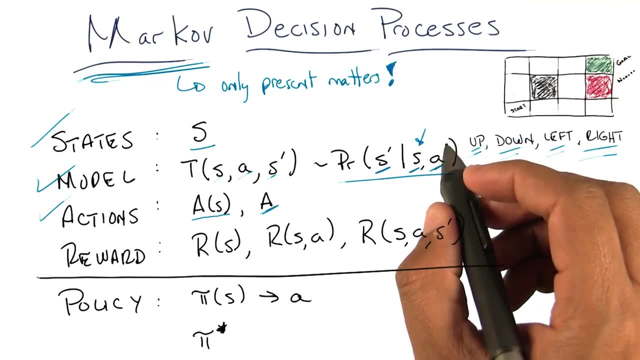 So what does this mean? What this means is our transition function, Which tells you the probability you end up in some state S prime. given that you were in state S and took action A only depends upon the current state S. If it also depended upon where you were 20 minutes before, then you would have to have more S's here and then you would be violating the Markovian property. 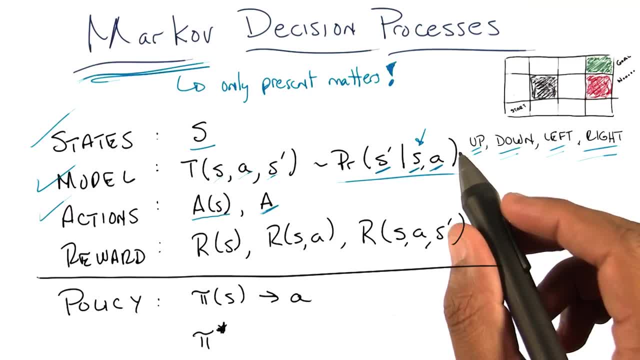 So is this like? do historians hate this? Well, you know, one never learns anything from history. No, you're supposed to learn from history or you're doomed to. I don't know. let me make something up, Repeat it. 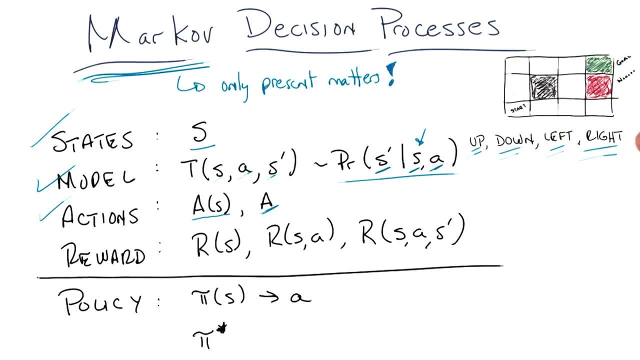 Fair enough. Historians probably don't like this, but there is a way for mathematicians to convince them that they're okay with it, And the way that you mathematicians convince you that you're okay with this is to point out that you can turn almost anything into a Markovian process by simply making certain that your current state remembers everything you need to remember from the past. 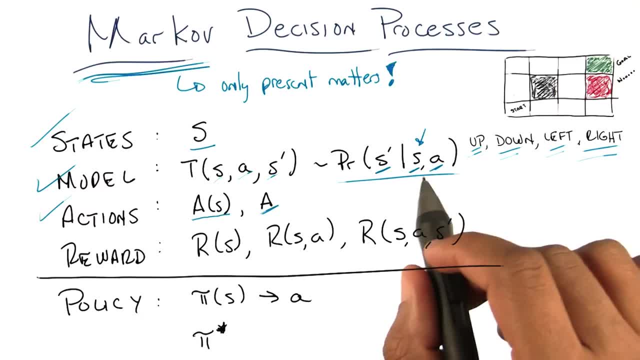 I see. So, in general, even if something isn't really Markovian, you need to know what you're, not only what you're doing now, but what you were doing five minutes ago. You could just turn your current state into what you're doing now. 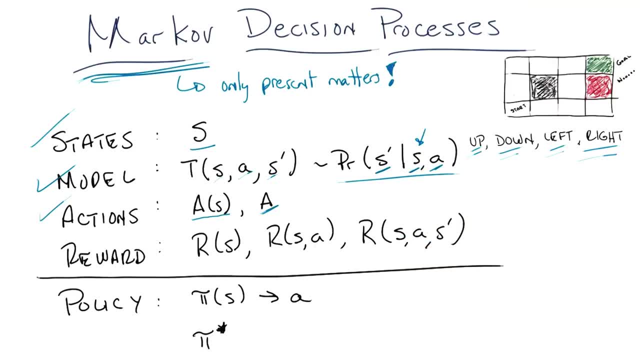 I see, And what you were doing five minutes ago. The obvious problem with that, of course, is that if you have to remember everything from the beginning of time, you're only going to see every state once and it's going to be very difficult to learn anything. 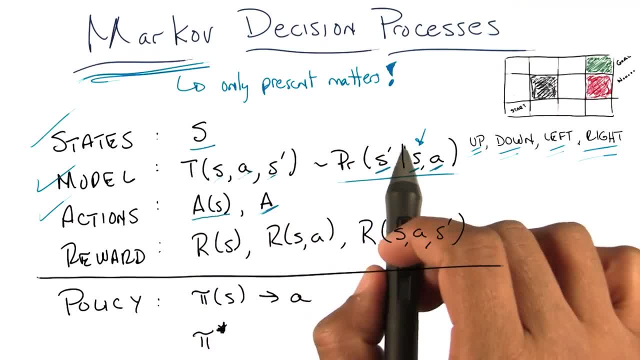 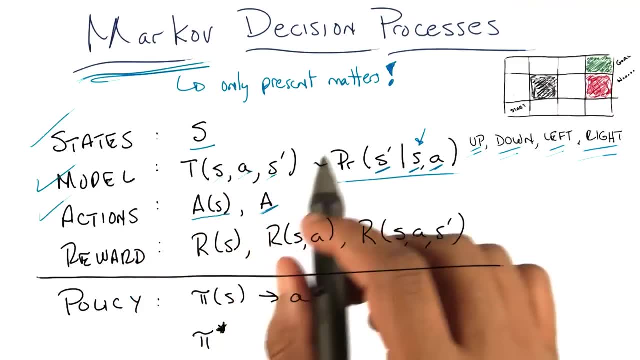 But that Markovian property turns out to be important and it actually allows us to solve these problems in an attractable way. But I snuck in something else, Michael. What I snuck in is this idea about the transition model: is that nothing ever changes? 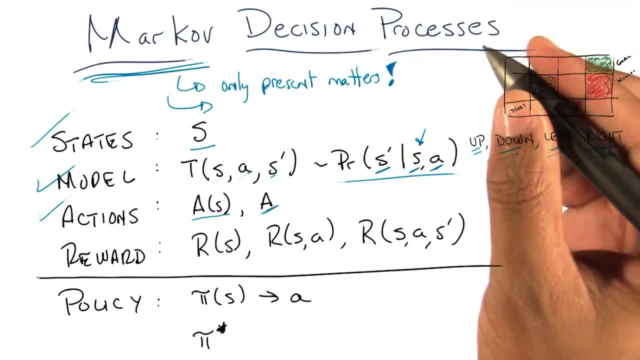 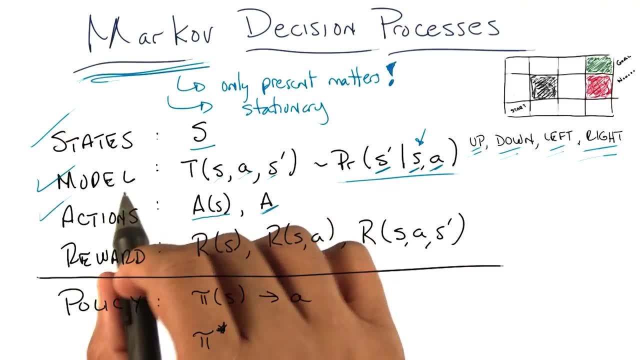 So the second property that matters for Markov decision processes, at least for the sets of things that we're going to be talking about in the beginning, is that things are stationary. That is these for the purposes of this discussion. it means that these rules 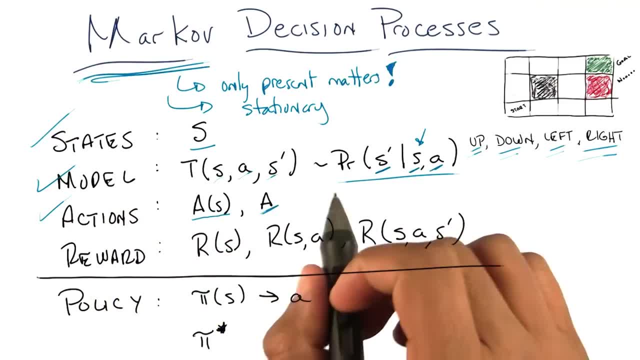 don't change over time. That's one notion of stationary. Okay, Does that mean that the agent can never leave the start state? No, the agent can leave the start state anytime. it takes the action that gets it out of the start state. 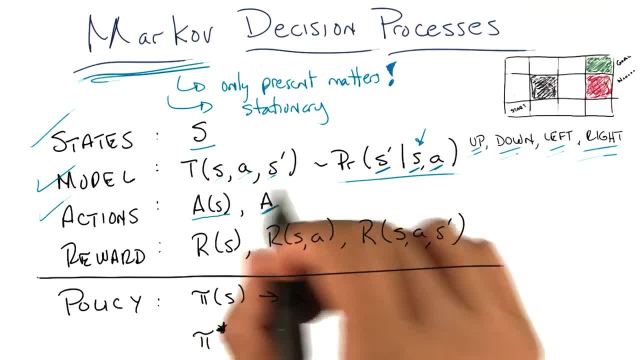 How is it stationary then? It's not stationary. The world is stationary, The, the transition model, is stationary, The physics are stationary. The rules don't change on you. The rules don't change, Right, Okay, okay, I see. 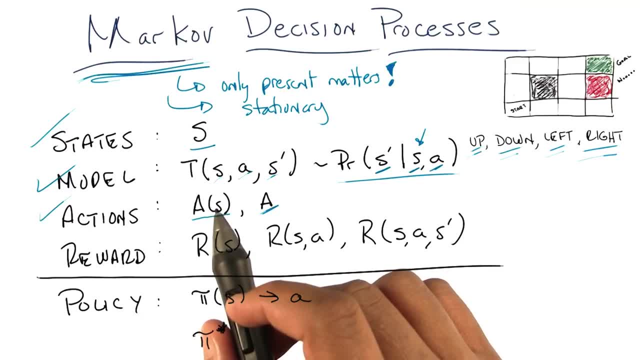 There's another notion of stationary that we'll see a little bit later. Okay, last thing to point out about the definition of a Markov decision process is the notion of reward. So reward is simply a scalar value that you get for being in in a state. So, for example, we might say: you know. 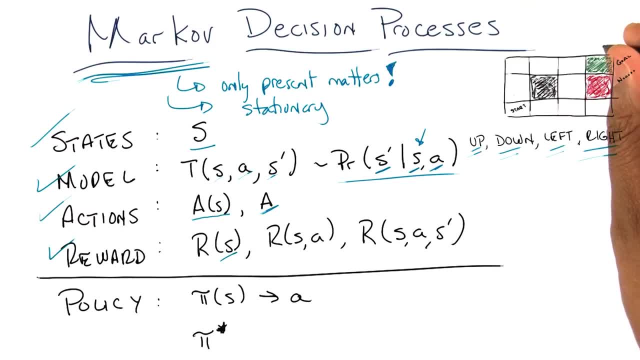 this green goal is a really good goal, And so if you get there, we're going to give you a dollar. This red goal, on the other hand, is a very, very bad state. We don't want you to end there, And so if you end up there, 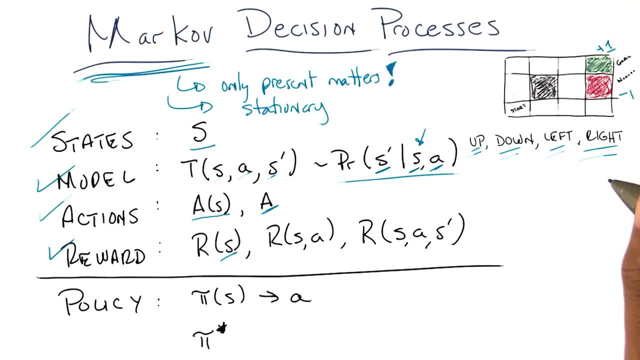 we're going to take away a dollar from you. What if I don't have a dollar? Someone will give you the dollar. The universe will give you the dollar. Or And then take it away. The universe will take it away Even if you don't have it. 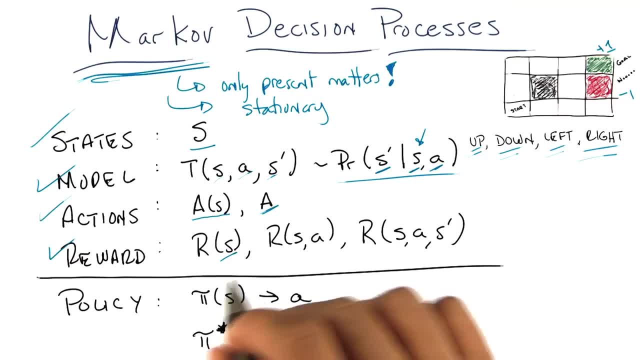 You'll have negative dollars, Oh man, Okay. So reward is very important here in a couple of ways. Reward is one of the things that, as I'm always harping on, encompasses our domain knowledge. So the reward you get for an estate tells you the usefulness of entering into that state. 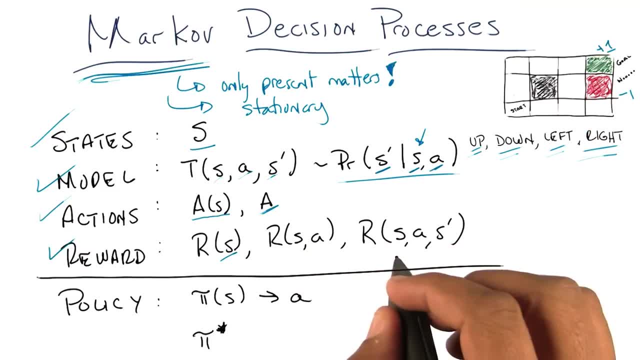 Now I wrote out three different definitions of the state and there are a number of them- different definitions of R- here, because sometimes it's very useful to think about them differently. I've been talking about the rewards you get for entering into the state, but there's also a notion of reward that you get for entering. 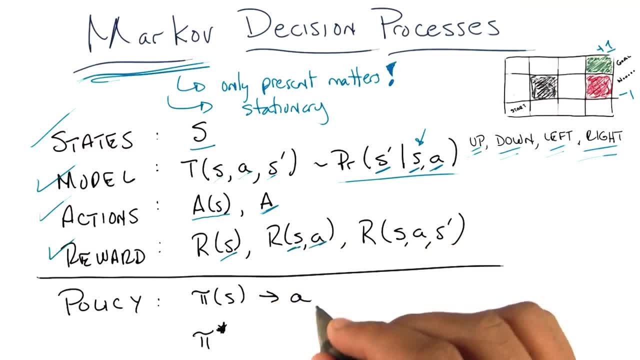 into a state and taking an action, There's a reward. or being in a state and taking an action, There's a reward that you could get for being in a state, taking an action and then ending up in another state as prime, It turns out. 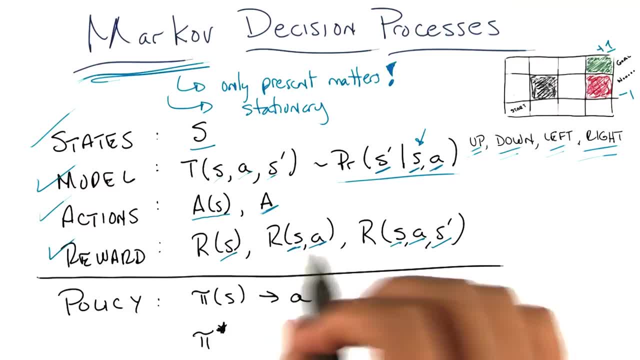 these are all mathematically equivalent, but often it's easier to think about one form or the other. But for the purposes of the, you know, for the rest of this discussion, really, you can just focus on this one, The reward, or 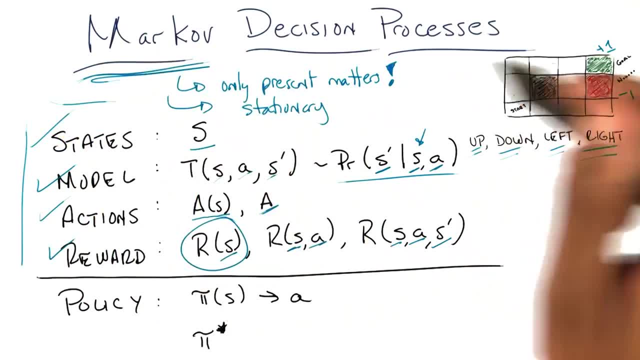 the value of entering into a state, And those four things by themselves, along with this Markov property and non-stationarity, defines what's called a Markov decision process, or an MDP Got it. I'm a little stuck on the how those could be mathematically equivalent. 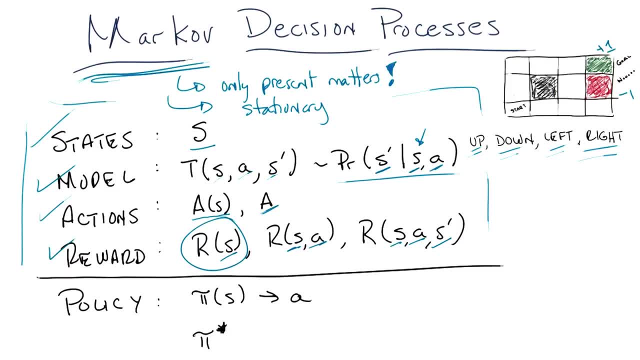 Well, we'll get to that later. Do you like a little bit of intuition? Sure, Well, you can imagine that, just as before we were dealing with the, the notion of making a non-Markovian thing Markovian, by putting a little bit of history into your state, you can always fold in the